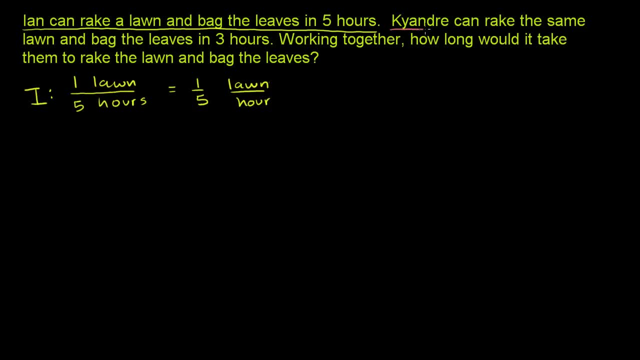 Now let's do the same thing for Keandre. Keandre can rake the same lawn and bag the leaves in three hours. So for Keandre, Keandre can for one lawn- I'll assume it's a boy's name- he can do it in three hours. 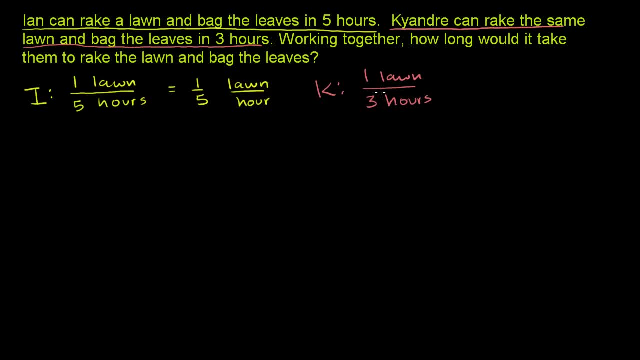 Or if we were to write it as a rate, this is 1 third of a lawn per hour. Now let's think about what the combined rate is. So let's say, if we have Ian plus Keandre, What's going to be their combined rate? 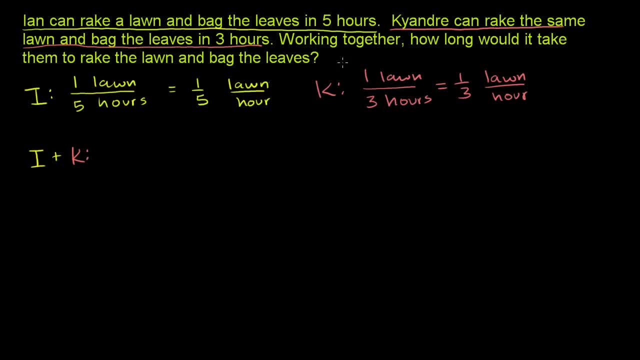 Well, they tell us that working together, how long would it take them to rake and bag the leaves? So let's let t be how long it will take them together. So that's how long they would take together. And if we say t is how long they take together, 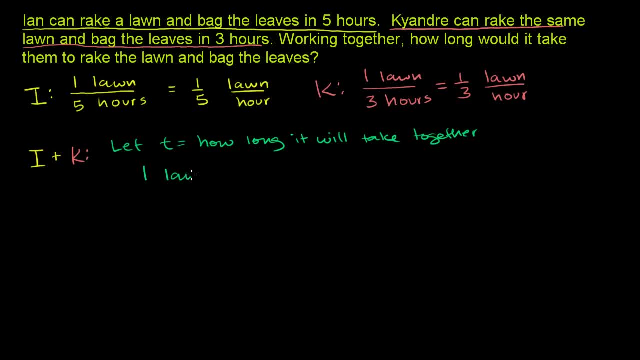 then we could say that combined they will do one lawn in every t hours. If we're assuming t is in hours for every t hours Or as a rate, their combined rate is going to be 1 third of a lawn per hour. 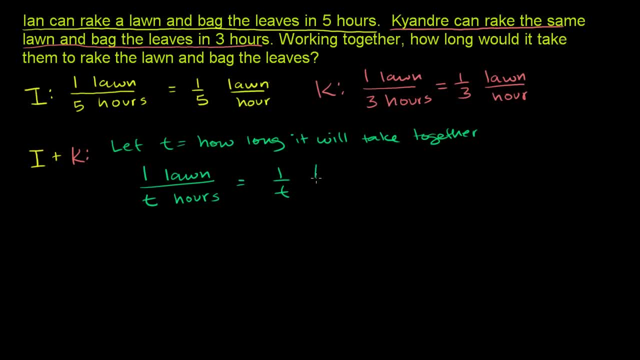 OK, 1 over t, 1 teeth of a lawn per hour, 1 over t lawns per hour. So that's their combined rate. So here we have the rate of Ian and the rate of Keandra and the combined rate. 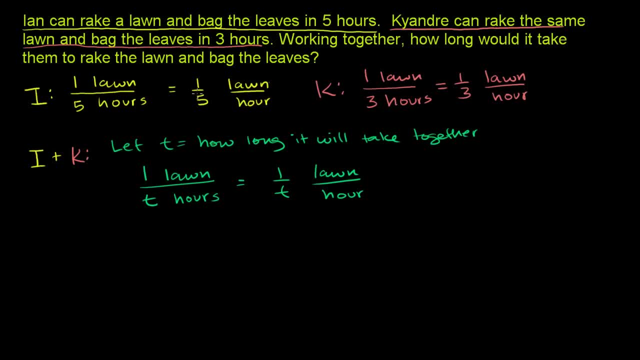 So the combined rate is just going to be the sum of each of their rates. If he can do 1 fifth of a lawn per hour and he can do 1 third of a lawn per hour, their combined rate is going to be 1 fifth of a lawn per hour. 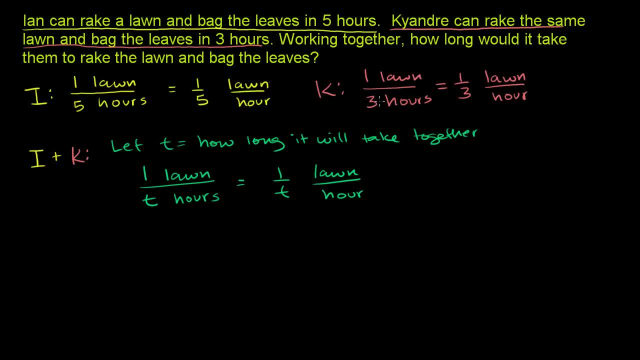 plus 1 third of an hour, Because in an hour he'll do 1 fifth and he'll do 1 third. So you'll add those two together to figure out how much they can do in an hour. So their combined rate is going to be 1 fifth lawn per hour. 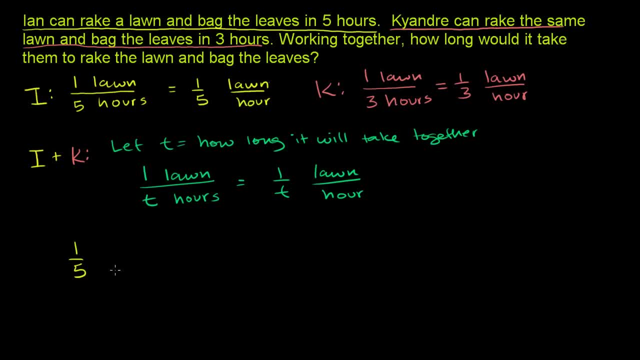 And I won't write the units here, just because it gets redundant. 1 fifth lawn per hour I could write over here, plus 1 third lawn per hour for Keandrae, Plus 1 third of a lawn per hour for Keandrae. 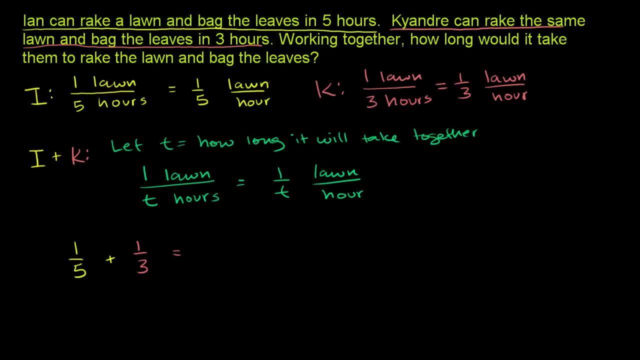 That's going to be their total rate, which is 1 over t lawns per hour, And now we just have to solve for t And we'll know the total rate, The total number of hours it will take them. So let's do that. 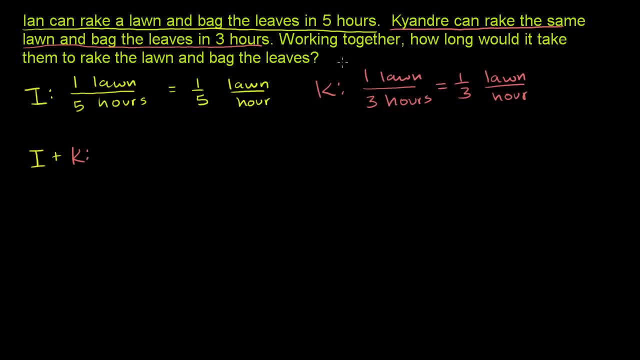 Well, they tell us that, working together, how long would it take them to rake and bag the leaves? So let's let t be how long it will take them together, How long it will take together. So that's how long they would take together. 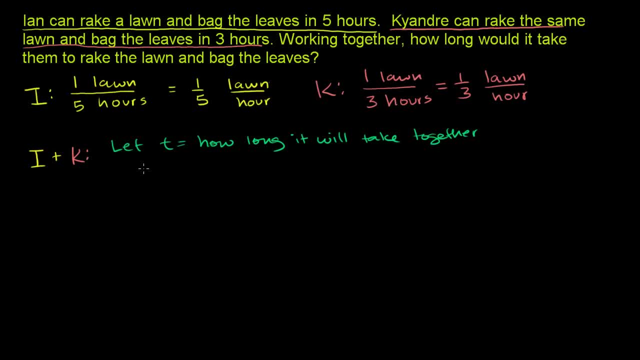 And if we say t is how long they take together, then we could say that combined they will do one lawn in every t hours. if we're assuming t is in hours For every t hours Or as a rate, their combined rate. 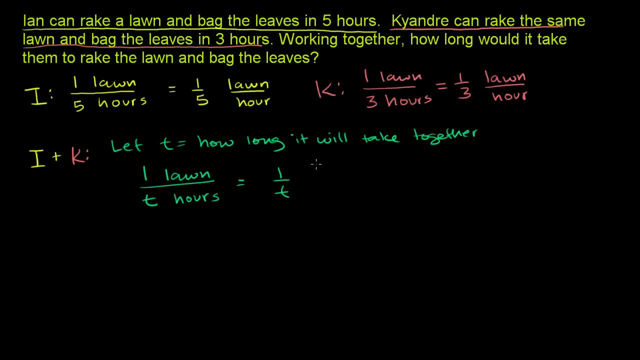 is going to be 1 over t, 1 teeth of a lawn per hour, 1 over t lawns per hour. So that's their combined rate. So here we have the rate of Ian and the rate of Keandre and the combined rate. 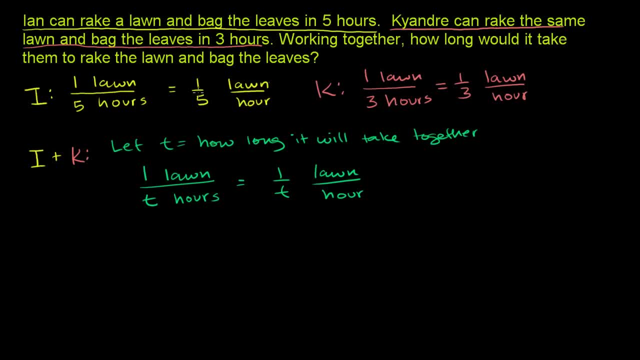 So the combined rate is just going to be the sum of each of their rates. If he can do 1 fifth of a lawn per hour and he can do 1 third of a lawn per hour, their combined rate is going to be 1 fifth of a lawn per hour. 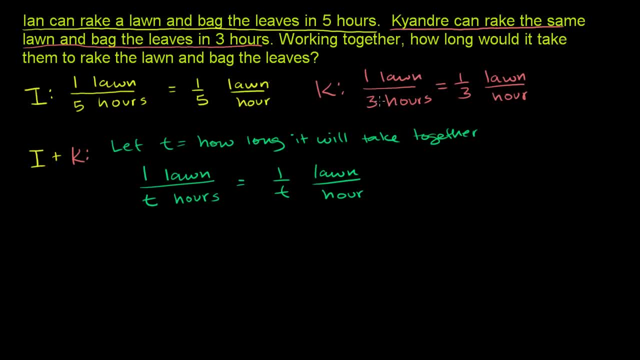 plus 1 third of an hour, Because in an hour he'll do 1 fifth and he'll do 1 third. So you'll add those two together to figure out how much they can do in an hour. So their combined rate is going to be 1 fifth lawn per hour. 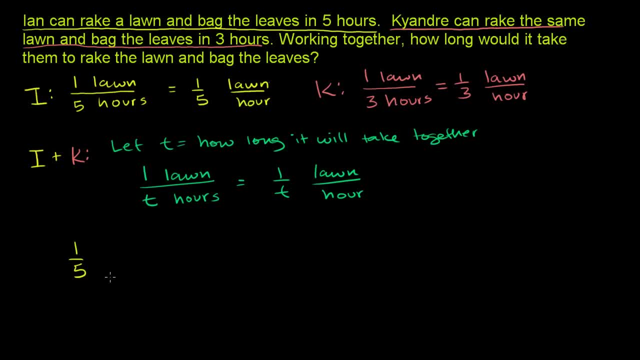 And I won't write the units here, just because it gets redundant: 1 fifth lawn per hour I could write over here, plus 1 third lawn per hour for Keandre, Plus 1 third of a lawn per hour for Keandre. 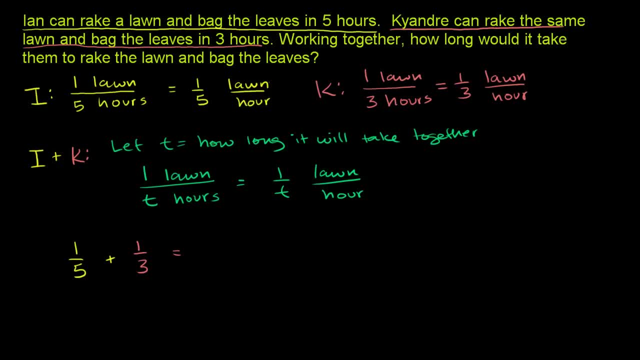 That's going to be their total rate, which is 1 over t lawns per hour. And now we just have to solve for t And we'll know the total number of hours it will take them. So let's do that. So to do that, we just have to add 1 fifth plus 1 third. 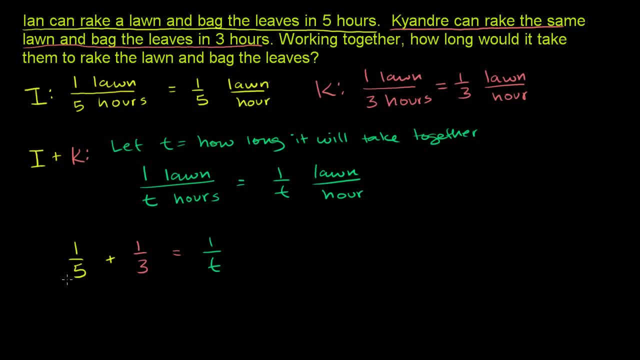 So to do that, we just have to add 1 fifth plus 1 third. Well, we can have a common denominator of 15.. So this is the same thing as 3 over 15, plus 5 over 15 is going to be equal to 1 over t. 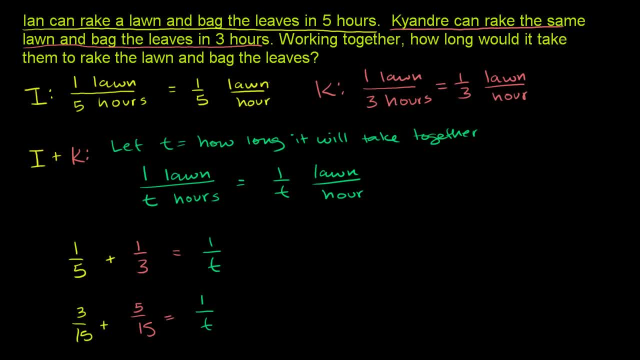 And then we have a common denominator now. So 3 plus 5 is 8.. So this is going to be 8 over 15.. I'll go over here now. So now we have, 3 plus 5 is 8 over 15 is equal to 1 over t. 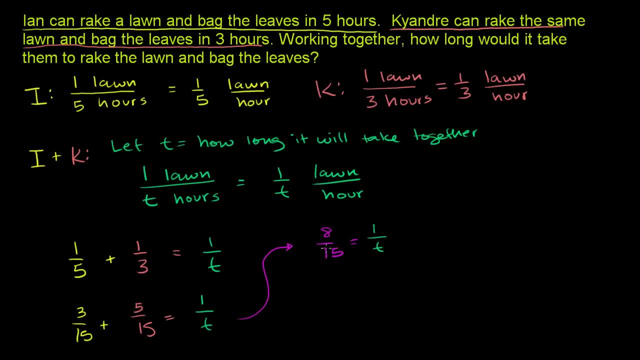 If we want to solve for t, we could take the reciprocal of both sides. So if we flip the left side, we get 15 over 8. And if we flip the right side we get t over 1, or just t. 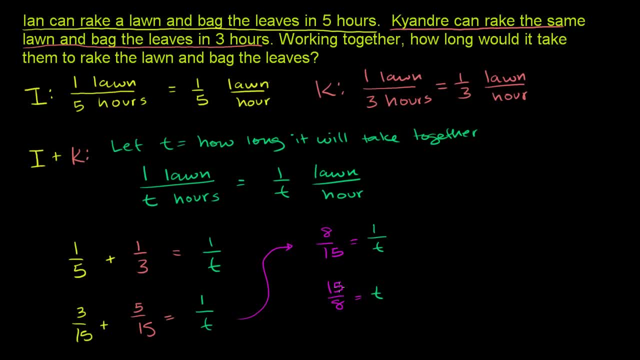 So it'll take them 15 over 8 hours or, if we want that in kind of a way that we can think about it a little bit better, 15 over 8.. So t? t is equal to 15 over 8 hours. 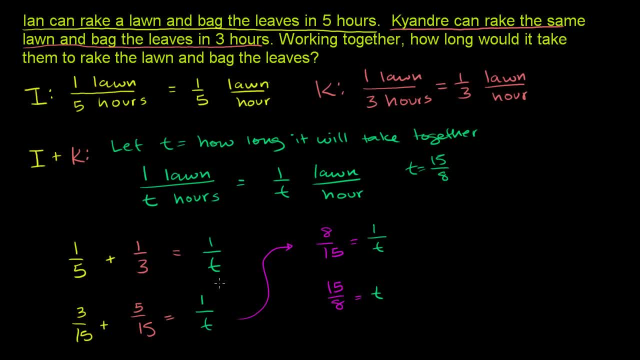 And I should say 15 over 8 hours per lawn. This whole time. here we had lawns per hour, This was lawns per hour, This was lawn per hour And this was here as well, lawns per hour. When we flip it, it becomes hours per lawn. 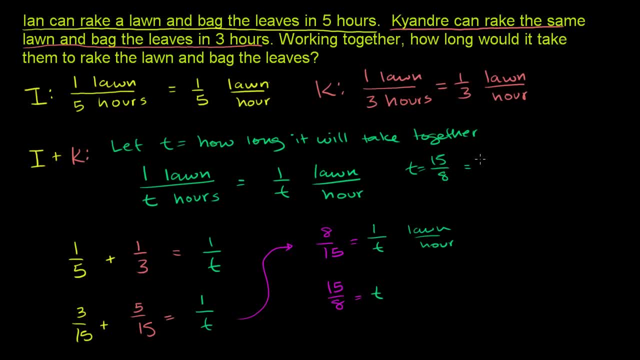 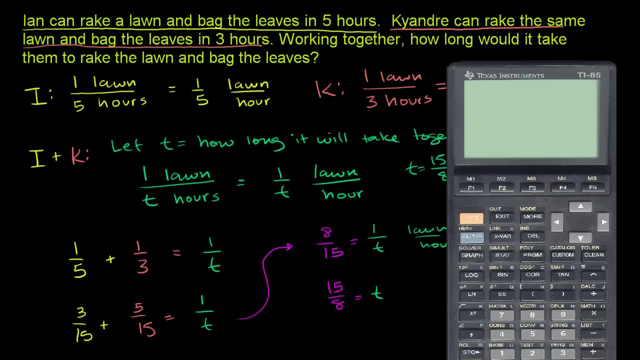 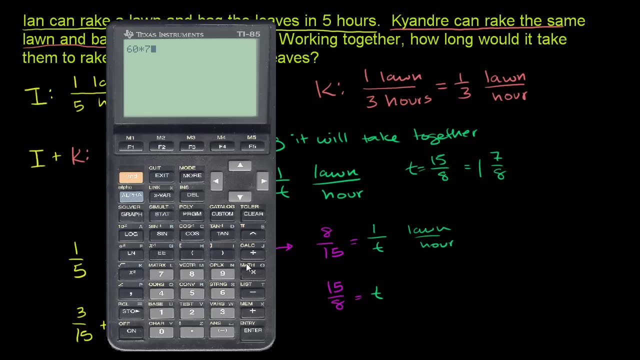 So that's exactly what we want. But 15 over 8 is the same thing as 1 and 7 eighths hours And 7 eighths of an hour. we can get our calculator out If we have 60 minutes in an hour times 7 eighths. 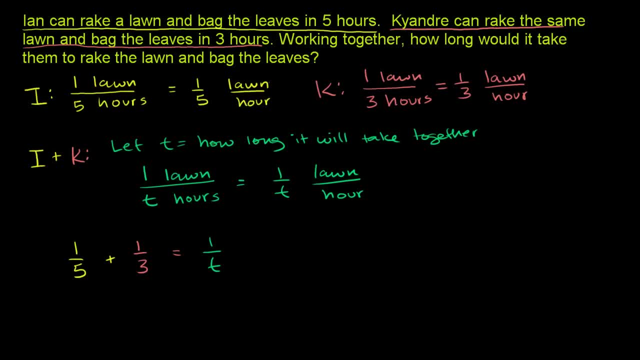 Well, we can have a common denominator of 15.. So this is the same thing as 3 over 15, plus 5 over 15 is going to be equal to 1 over t, And then we have a common denominator now, So 3 plus 5 is 8..